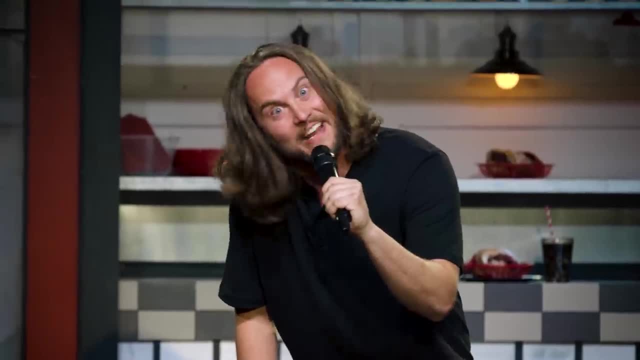 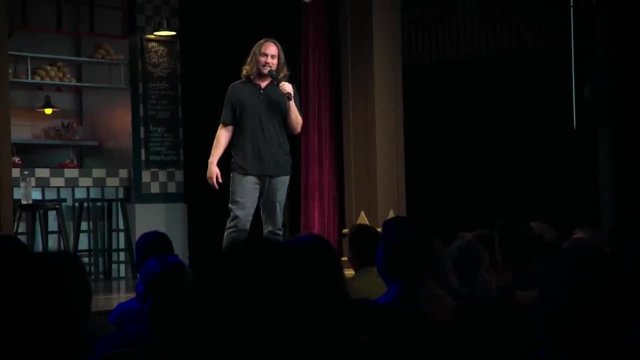 You want to go out? There's a tree. I know this tree. You want to hang out? There's a tree. What if I just keep breathing into your face All the time? No, thank you. That's why I like cats. Cats are more like: hey, what are you up to? 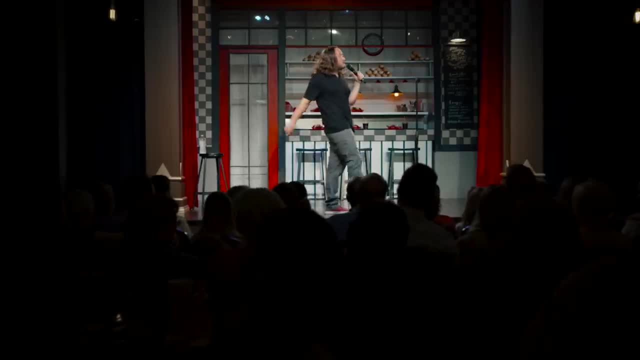 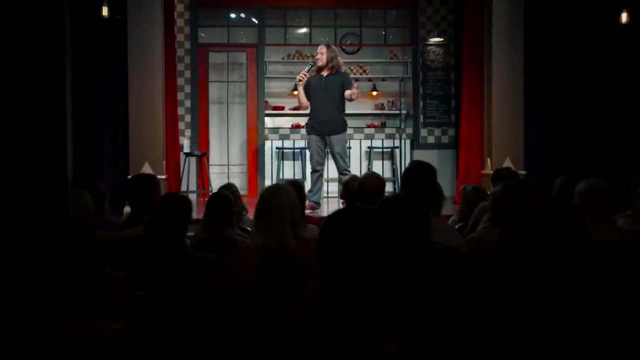 Never mind, I just remembered. I don't care, I'll be in the kitchen, I'll see you later. I like that. I don't need a best friend at the house, I just need, like, an apathetic roommate that sometimes wants to hang out. 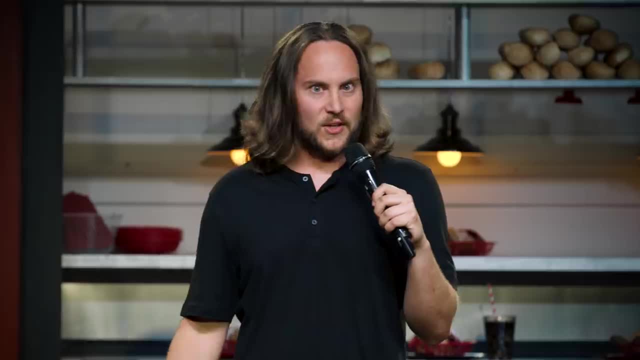 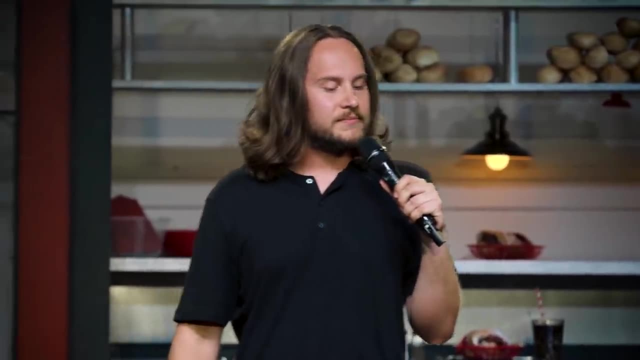 Like a dog. You can pet a dog All day, They'll never get tired of it. Just all day, Just like, yeah, man, never stop, You're the best. Hopefully not that creepy, but you get the idea. A cat you can pet for what Two? 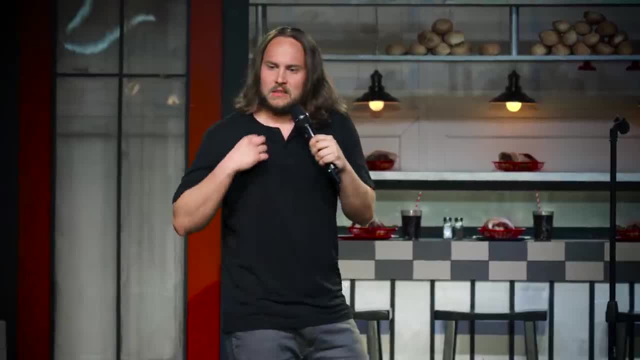 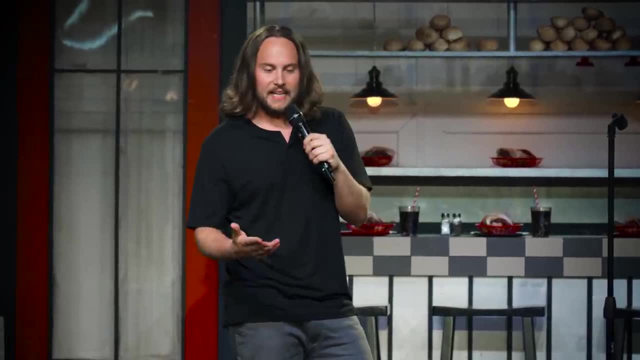 maybe three seconds, And so it's like: all right, get away from me. All my own things going on, I got a pile of clean laundry to lay on. Get away from me. That's what my cat does. It waits for the. 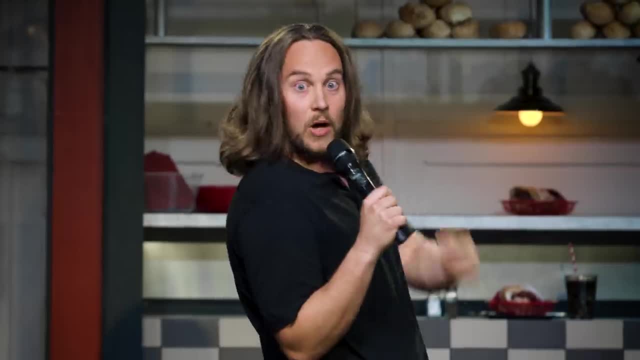 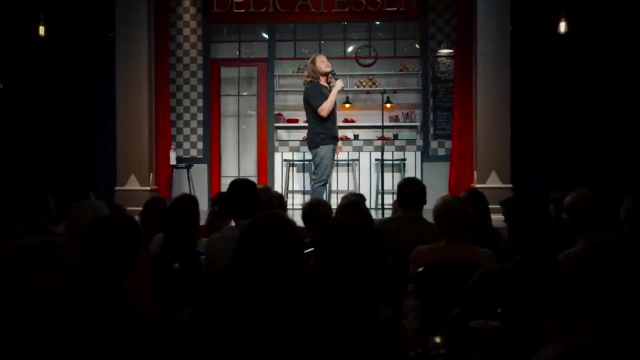 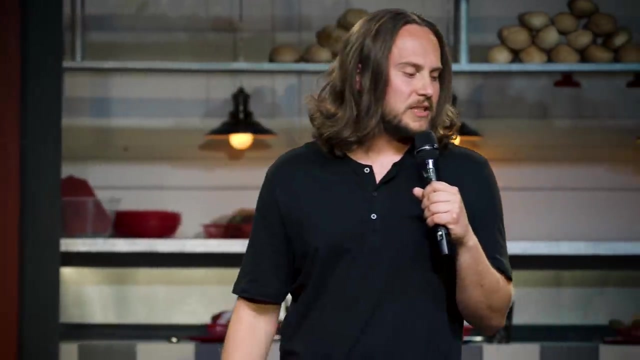 pile of clean laundry we haven't folded yet and just rubs on it while making eye contact Just like mm-hmm. Everyone's going to know So bothersome. My wife: she has a new hobby. She's really into special needs animals. I don't know if that's made. 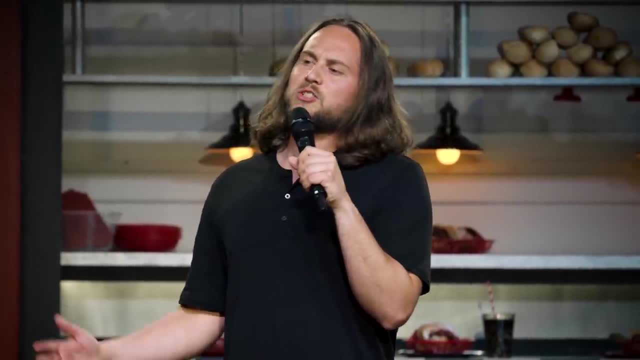 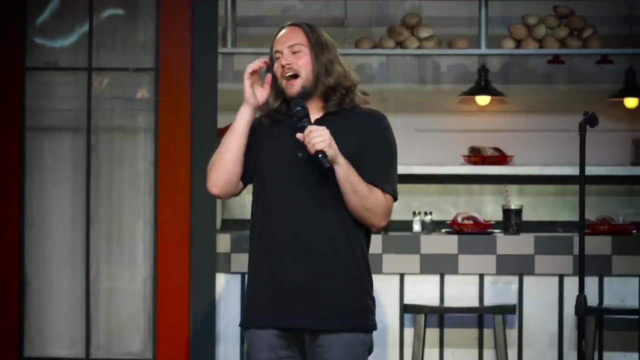 its way out here to Provo. If you don't know what special needs animals are, they're animals, They have special needs. That is all. There's this one, Oscar the blind cat. It was a cat that was born without any eyes And they have a like page And they have a like page And they have a. 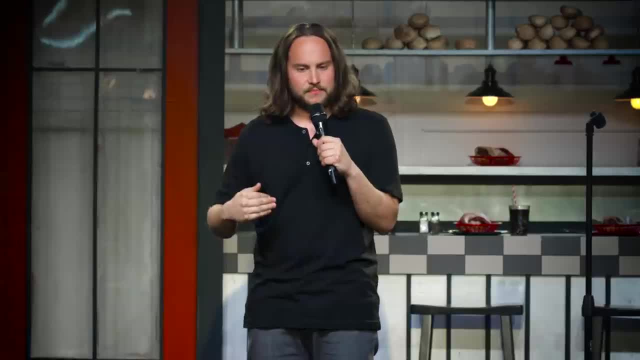 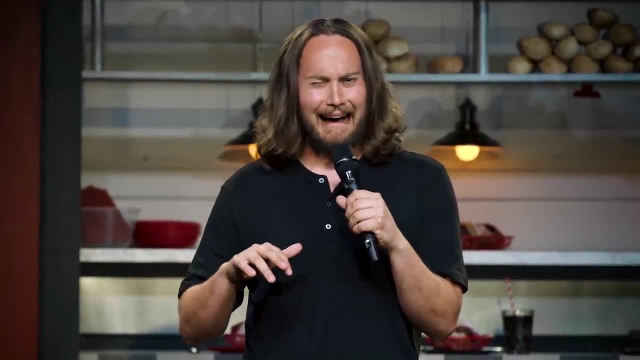 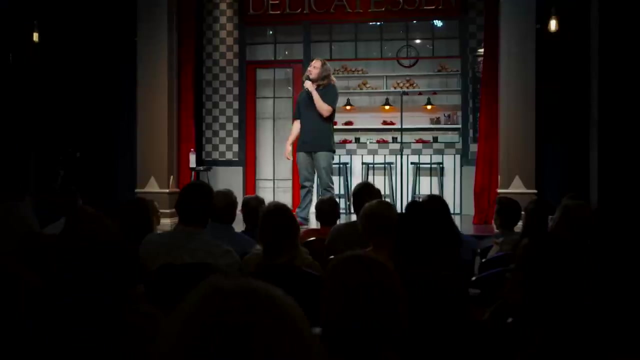 like page on Facebook And my wife goes on there every day and cries And that's what she does for fun, That's what she does for a good time. And it's weird because I come home and she's just on the computer And you know me being a guy, I always think it's something I did. And then she 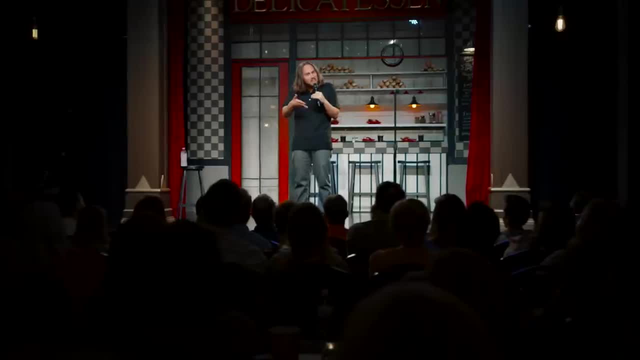 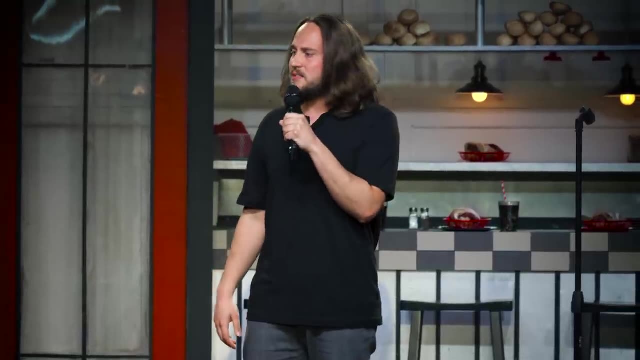 goes. no, And then she turns the computer and it's Oscar the blind cat. And you're like, look at Oscar And he's adorable, He has no eyes. And I'm like, oh, And then she goes, I want a special. 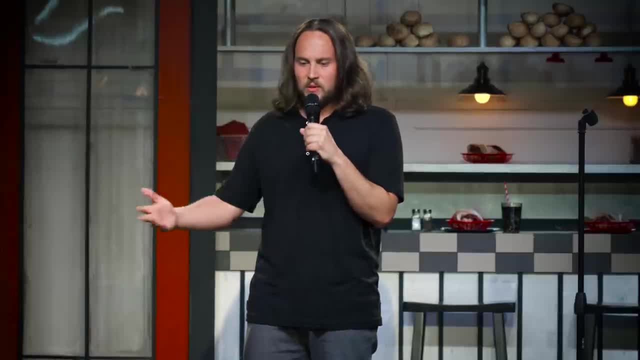 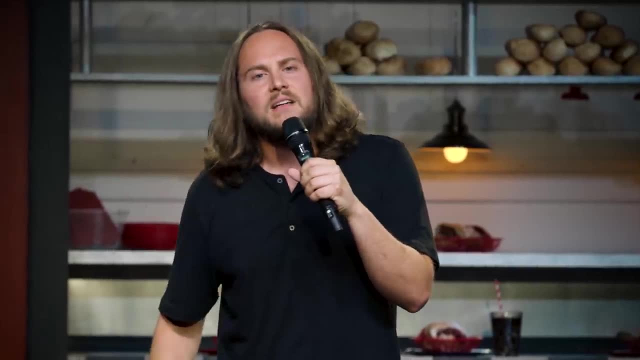 needs animal, I want one. I'm like you don't ask for one, You get bestowed one Because I don't know. You can't just go to the pound and be like, hey, what do you have in the back? Like that's. 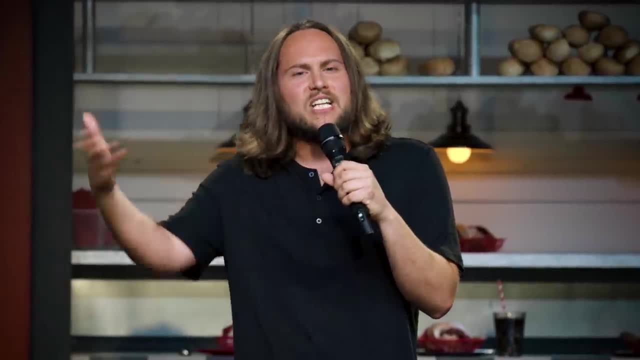 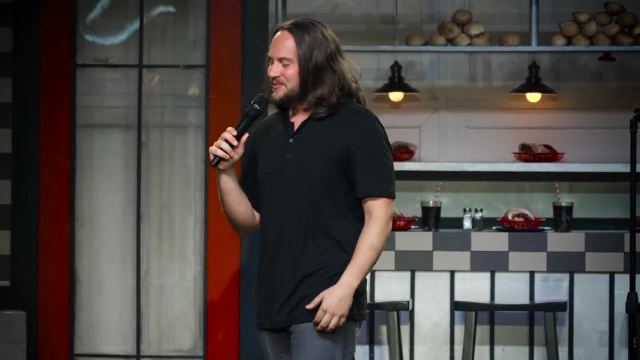 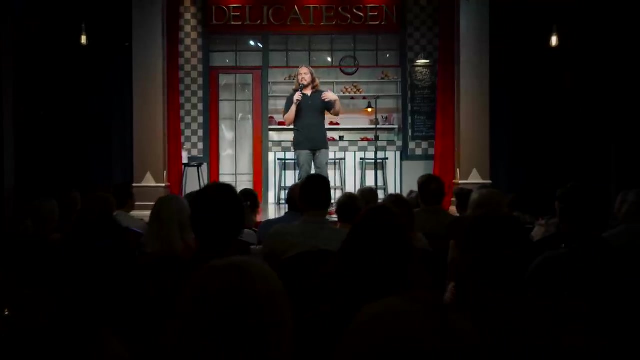 not how that works. I need like a three-legged dog or a cat with something. What do you have? I can't do that. That's why you know we got Jessica at the pound. That's where we got Jessica, And we didn't name her Jessica, They named her at the pound. 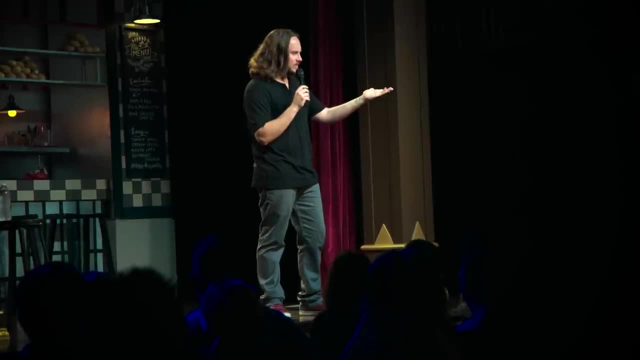 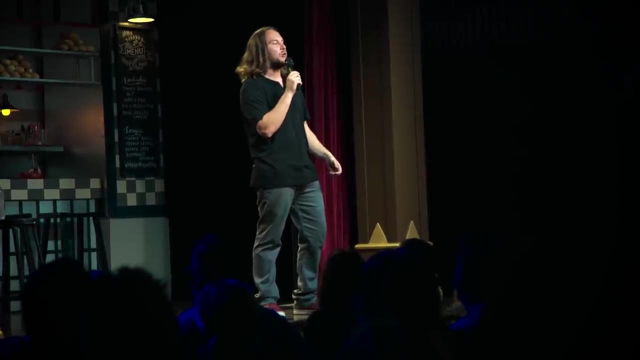 And people always ask, like: why don't you change your name? Because that's wrong. You don't change someone's name. That's rude, Like if you adopt a kid from another country, you can't just be like, yep, can't pronounce that Your name's Jeff. now, That's rude. You learned that person's name. 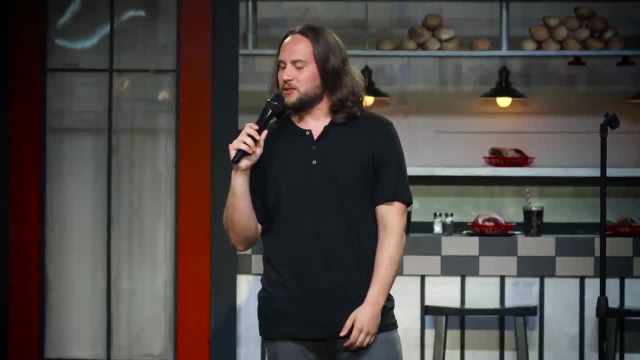 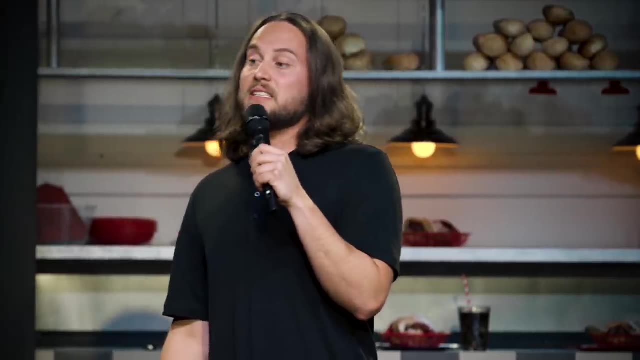 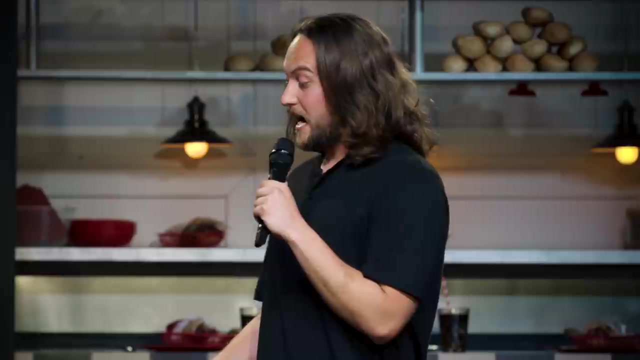 So I got a cat named Jessica. Very much your thing. Jessica's overweight. She weighs more than she should for a cat, Which sucks, Because when people come over, no one blames the cat. in that scenario, You know what I mean. No one comes over and goes. what happened here, sweetheart, A little heavy on. 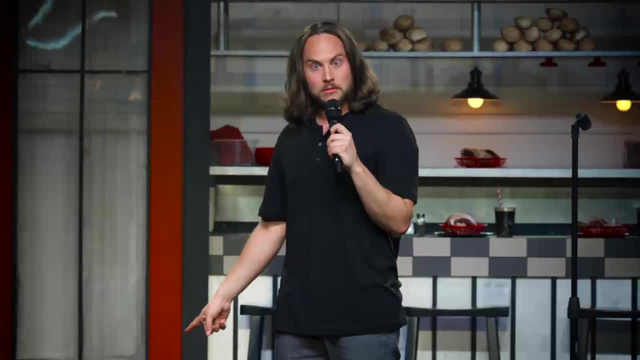 the carbs. No, they look at you and they go: what'd you do to her? And that's not fair. Because I try. We have the laser pointer. I got the stick with the feather I'm always running around my house. 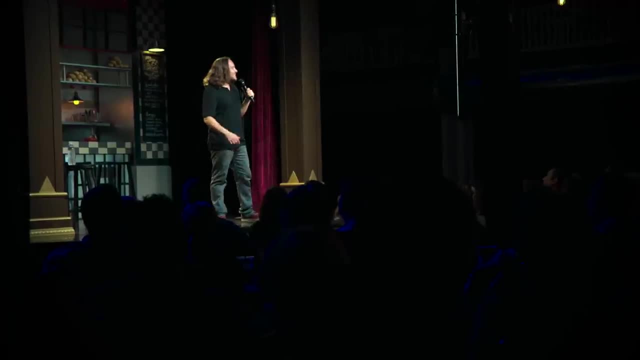 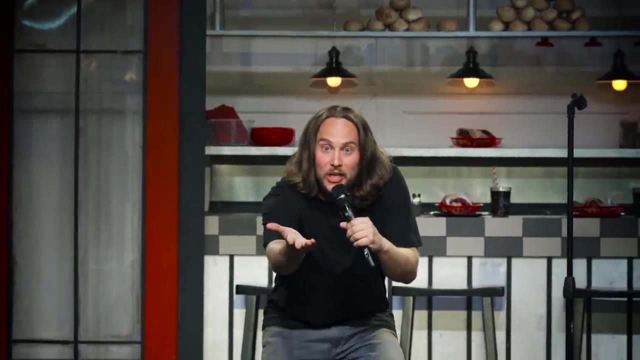 Come on, sweetheart, Let's get the cardio going. She's not that into it. My wife and I, we bought diet formula kibble. They make diet formula kibble And they have rules: Just one cup per day, Because you're on a diet, Jessica. 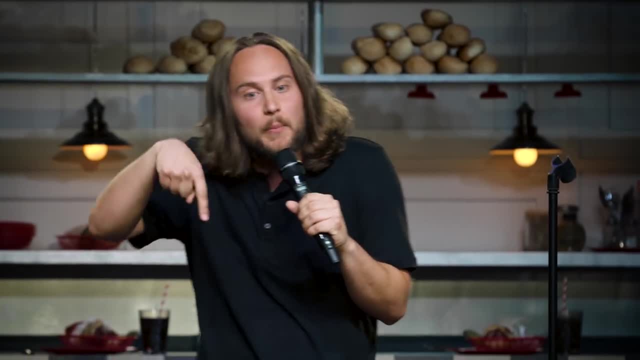 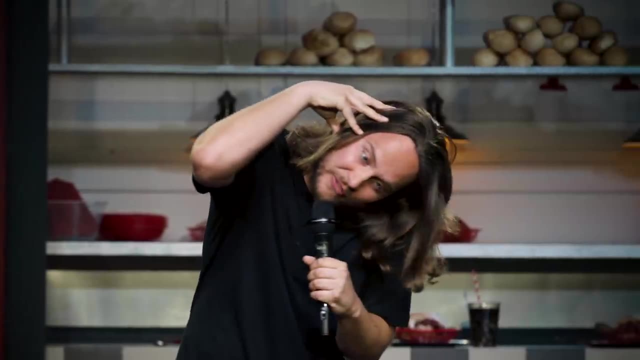 We tried, But then at two in the morning Jessica would come into our bedroom at night, climb onto our bed and then stand on my head- 22 and a half pounds of her, you guys, on my skull And she would come down into my ear and 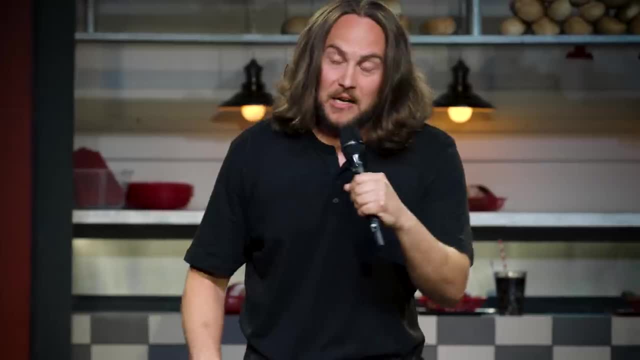 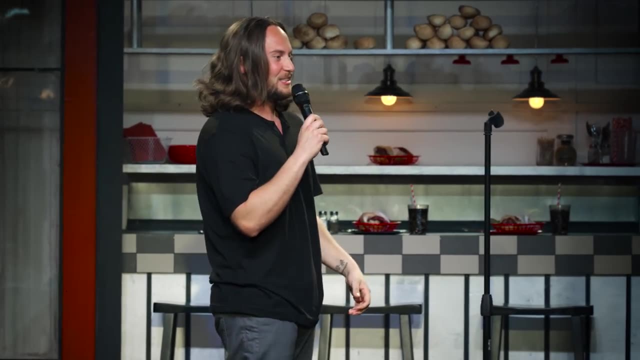 just go meh, meh And I'm like, yeah, you're right, This diet is over. I had no idea that's how you felt about it. I apologize. I am getting up right now and cooking you some bacon. 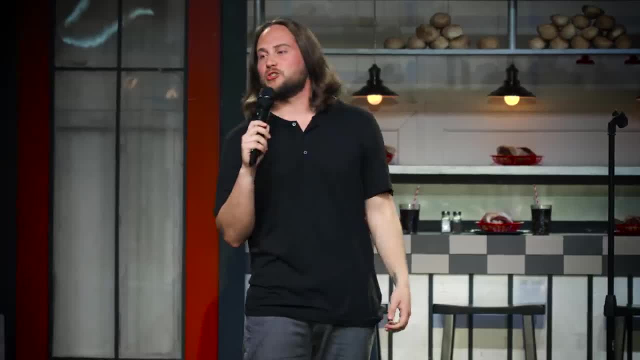 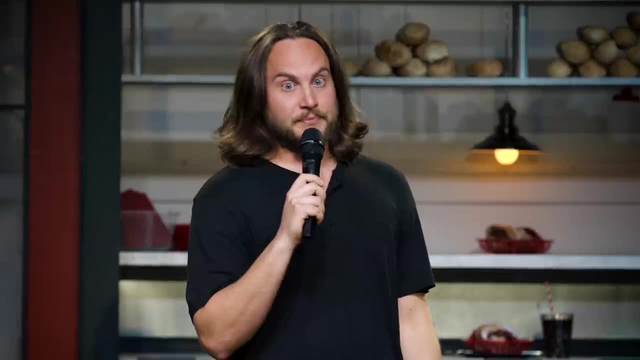 Let's get after it. I don't have any children, but if I'm out in public and I see a parent of an overweight child, I make eye contact and I go. I get it. Does that little fella stand on your head? 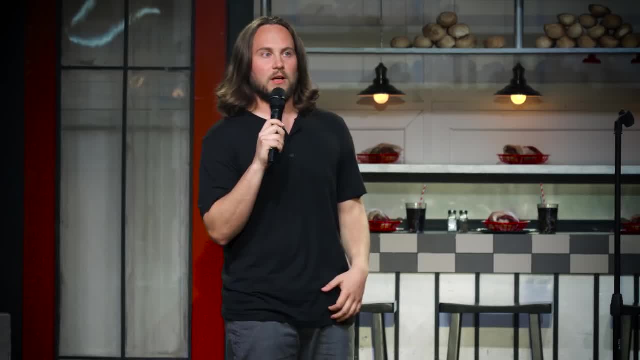 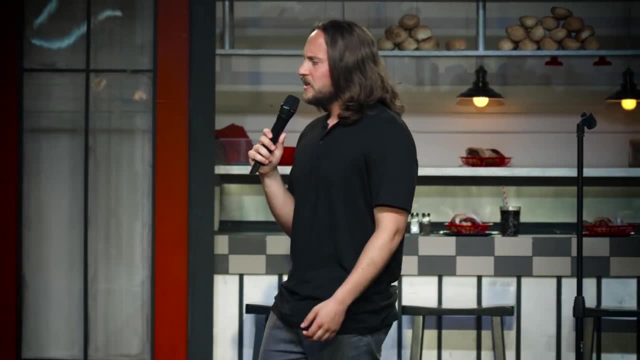 at night and scream in your ear. I get it. Give him what he wants. We need our sleep. My wife and I, we sleep on a memory foam mattress. That's what we sleep on. Anyone else here rocking the memory foam mattress? It's the best mattress in the world. It's the most comfortable, isn't it? 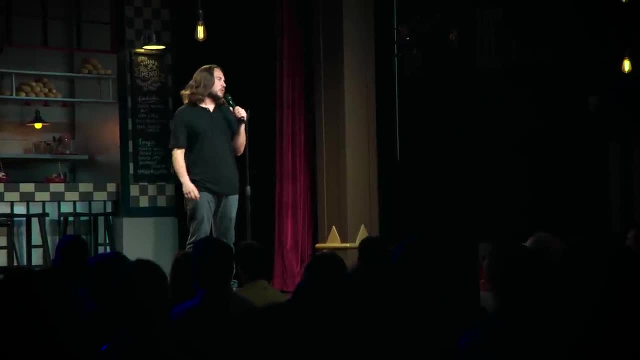 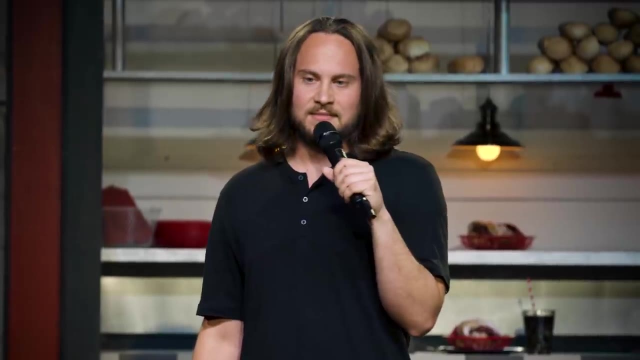 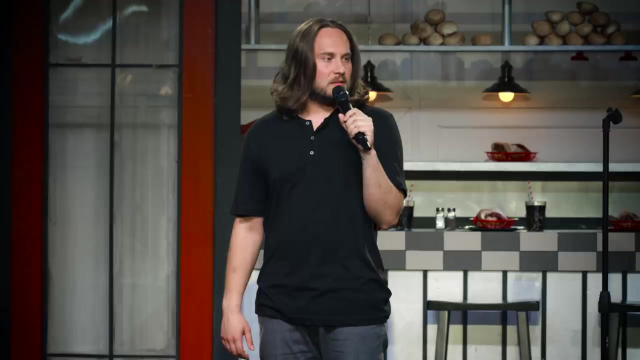 It's the best. That mattress is made for sleeping and sleeping only. Don't do anything else on that mattress. Who's not created for that? That is not why scientists came together. It's made for resting comfortably and that is it. I know because we've tried and it sucks every time. It's like trying. 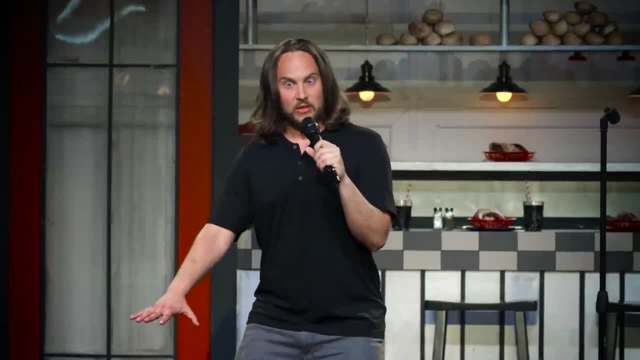 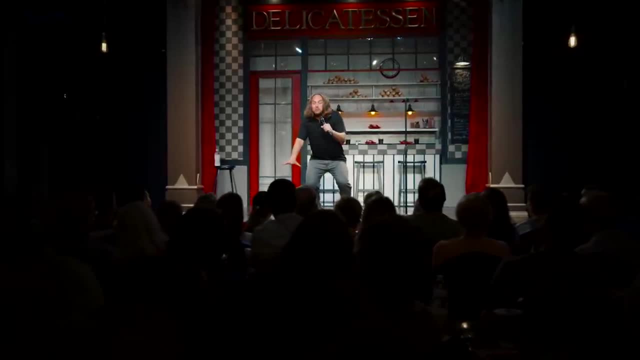 to wrestle in quicksand. It is the worst. You just start sinking in slowly. Stay calm, Stay calm. Just try to get your leg out. Just breathe, Keep your eyes open, Keep your eyes on the horizon, Try to get your leg out. Get your leg out, I'm going to get some. 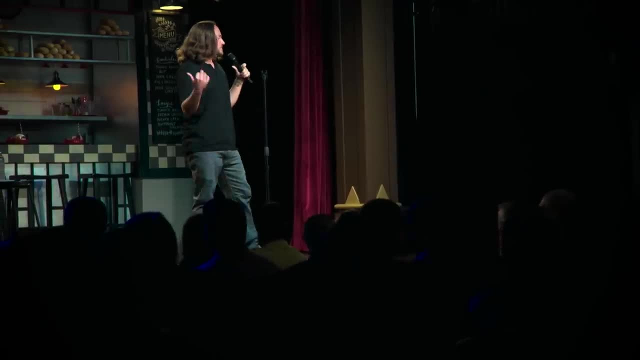 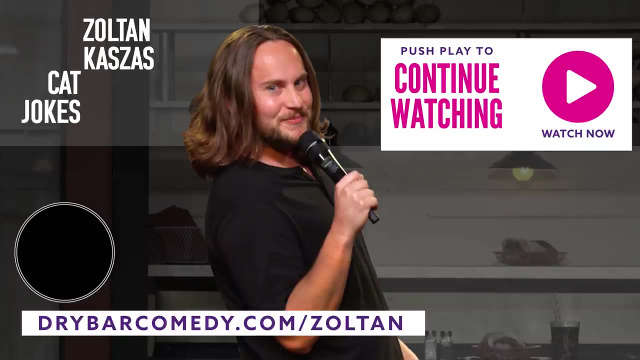 help Jessica. we need some help. She can't help, She just stands on our backs and pushes us in further. Subscribe to Dry Bar Comedy for even more of the world's largest collection of clean comedy. 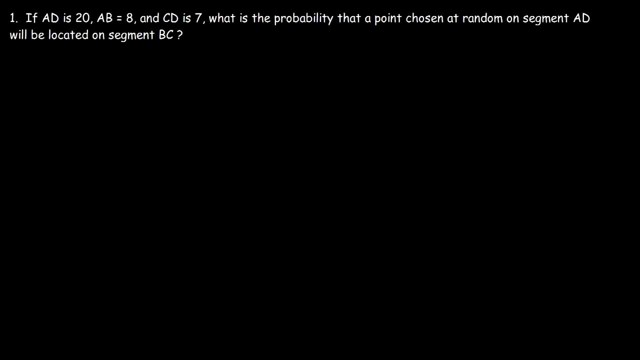 In this video we're going to talk about how to solve geometry probability word problems. So let's start with this example: If AD is 20,, AB is 8, and CD is 7,, what is the probability that a point chosen at random on segment AD will be? 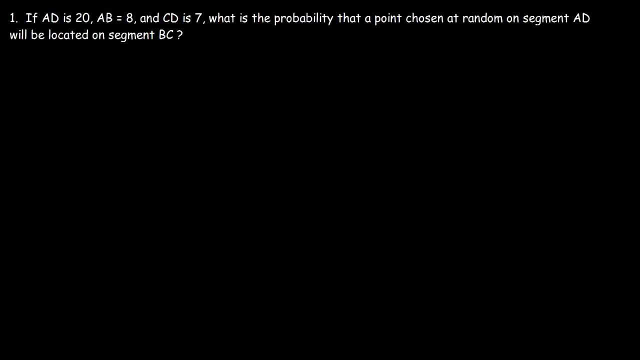 located on segment BC. And let's say in the picture that all the points are listed in alphabetical order. So this is point A and point D, And let's put B and C somewhere along this line. So we're told that AD is 20 units long and AB.